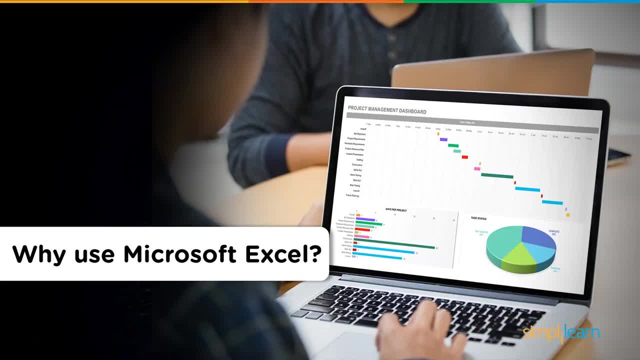 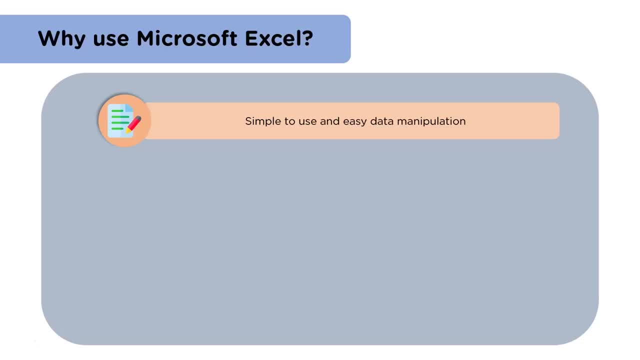 Before we learn more about project management in Excel, let's first have a look. why do we use Excel? Microsoft Excel is an easy tool to plan a project, so it can be used by people who are beginners in terms of project management. In Excel, one can find several analytical tools like concatenate, len and counter, so this makes data analysis easy and effective. 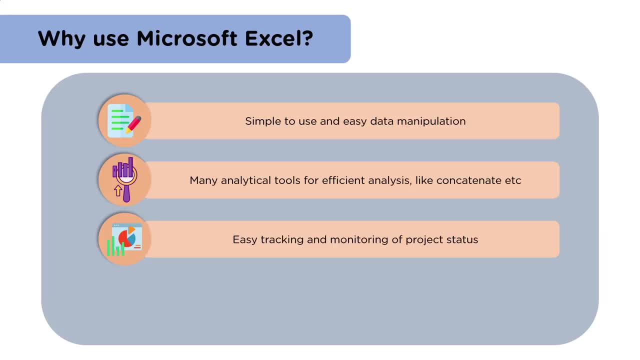 As the entry of data is easy, same is tracking and controlling of project status. Then there are several project management templates in Excel that help us to have an effective distribution of project data. We will be checking several project management templates towards the end of this video. 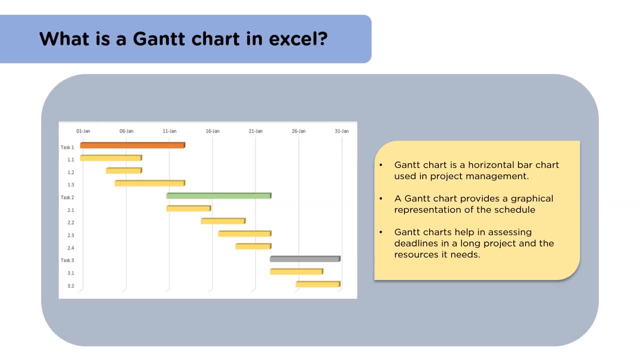 Now let's have a look at the process of making a Gantt chart in Excel. Before we begin this, it's important we know what is a Gantt chart. A Gantt chart is like a horizontal bar chart that is used for project management. 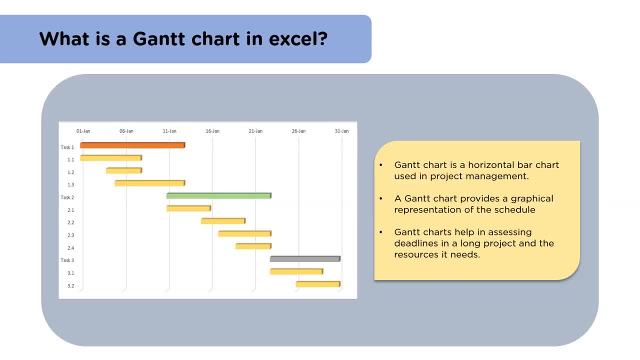 With the help of a Gantt chart, we can check the status of the task, the date they start, the date they end and their dependencies on each other. Gantt chart helps in coordinating and monitoring different tasks in a project. Now let's have a look at the steps that will help us in making a Gantt chart. 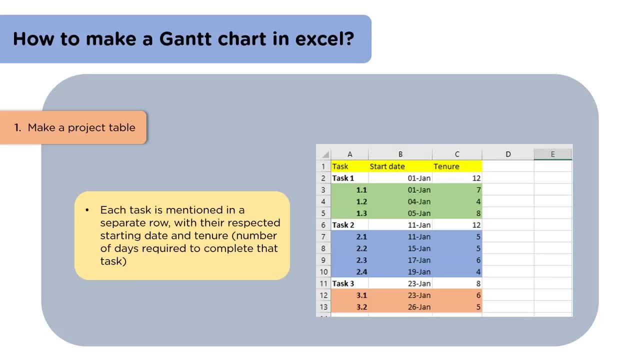 First step we have is make a project table. We have several rows and columns, Like here. we have three columns: In the first column we have the tasks, In the second we have our start date And in the third column we have the duration or tenure of the task. 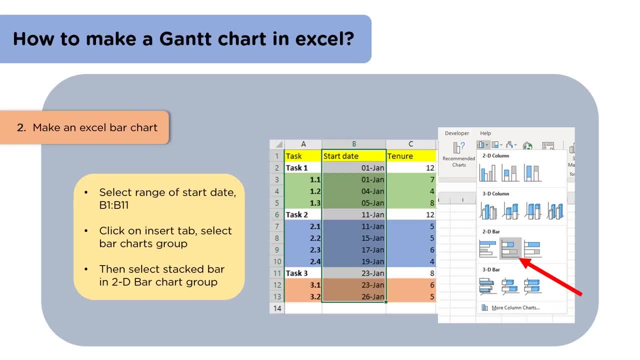 The second step is to make a bar chart in Excel. For this we will select the entire second column. Then we will go on the insert tab and click on the bar graph chart. There we can select stacked bar graph in 2D bar charts. 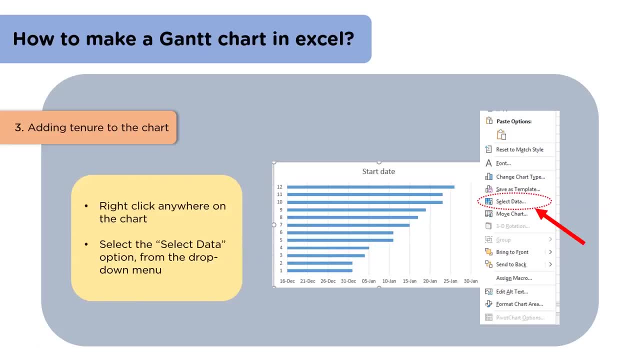 As a result, we will have the entitled bar graph on the screen. In the third step, we will add the duration to the bar graph. We will right click on the chart and in the menu that appears, we will select select data option. 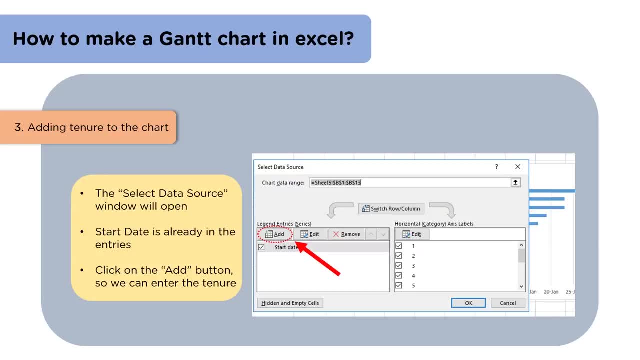 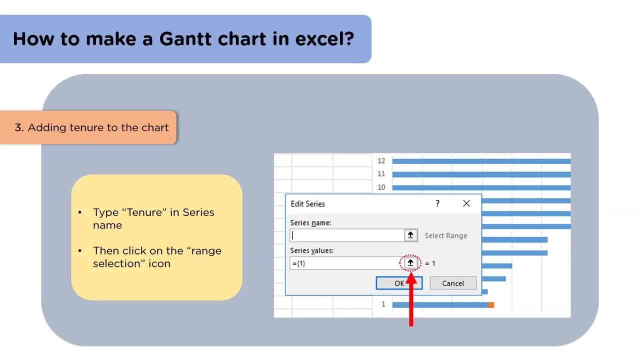 A window that appears on the screen. in that window we will select add option as shown. We can also see the start date is already in the entry section. Then in the dialog box that appears, type tenure in the series name and click on the range selection icon that's shown in the figure. 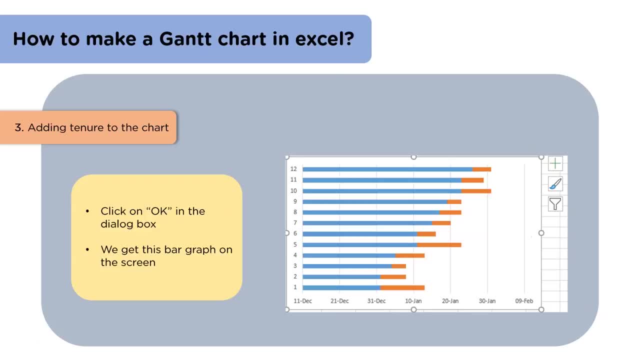 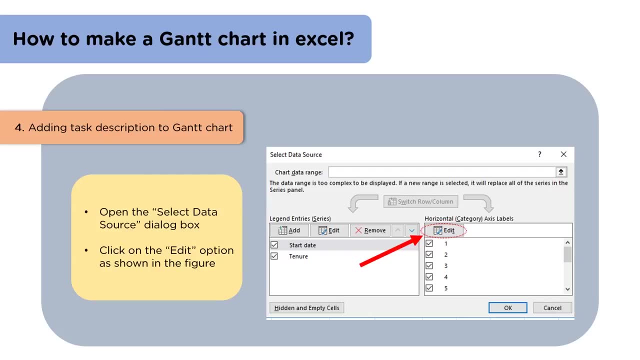 Now select the relevant data from the tenure column and click on OK. Now we can see a bar graph that has two colors on the screen. This bar graph now has the duration of the tasks. The fourth step we have is adding description to the Gantt chart. 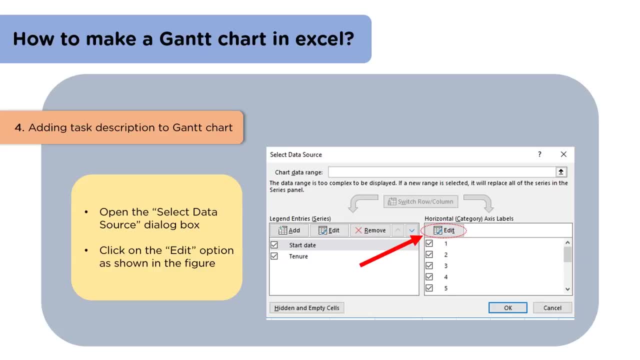 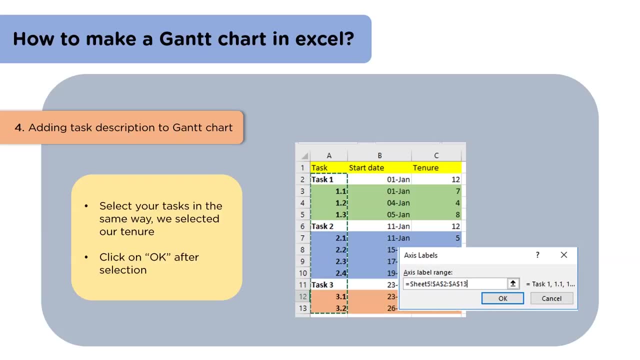 Now we will open the box again and in that box we will select the edit option as shown in the figure. Then we will select the tasks as we had selected the duration of the tasks before, and click on OK. We can now see the tasks have appeared towards the left side of the Gantt chart. 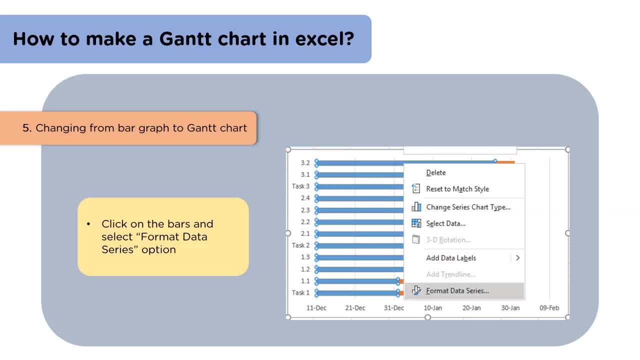 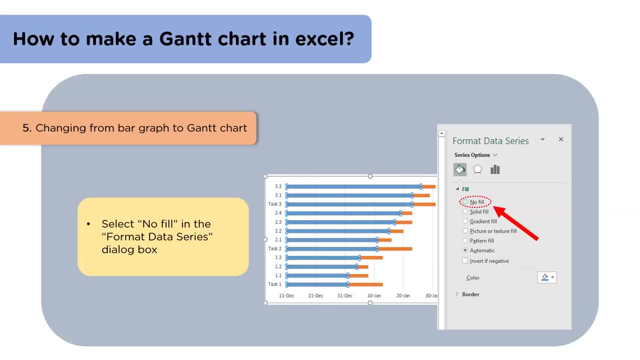 The fifth and the remarkable step will help us convert this bar graph into a Gantt chart. We will now click on the bars And select the format data series option from the menu that appears. Then in the format data series dialog box we will select no fill option. 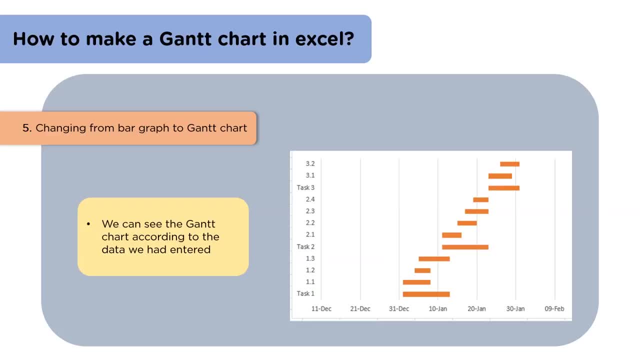 We can find our Gantt chart on the screen now, in accordance with the data that we had entered. Now we can see the tasks on the left side are in the reverse order, So what we will do next is we will click on the task panel. 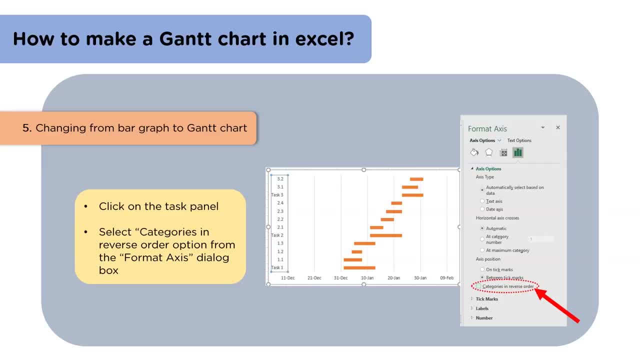 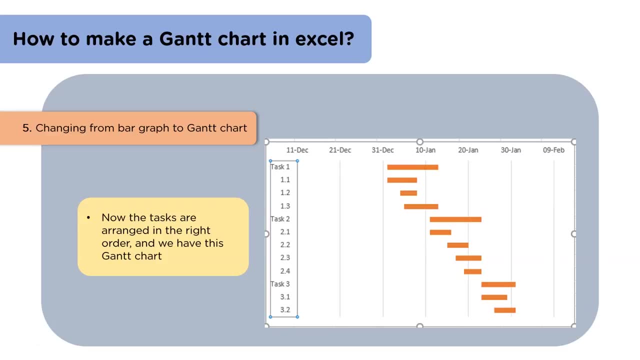 Then go to the format exercise dialog box and select the categories in reverse order option. Now we can find our tasks in the right order. One more thing we can notice is Gantt chart is starting with some other date and not with the dates that we had entered. 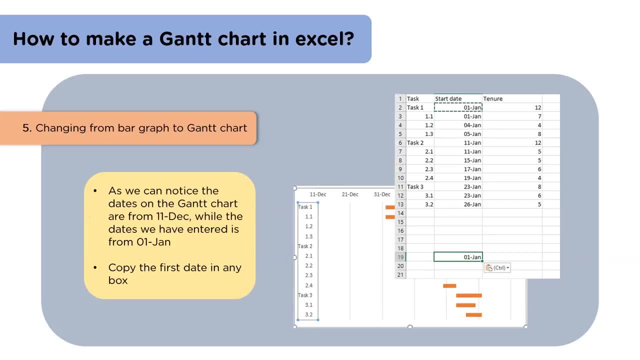 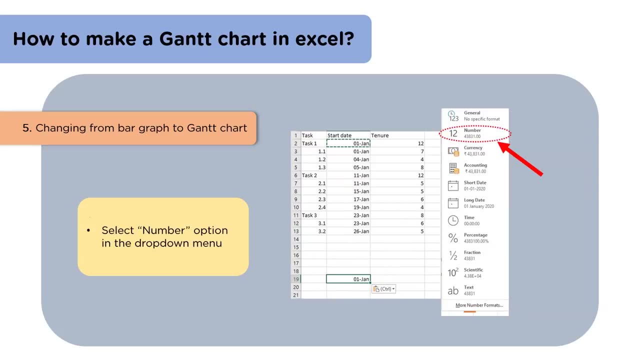 So for this we will copy the first date in some other cell. Then, clicking on the copied cell, we will go to the home menu to select the dialog box as shown in the figure. Then in that drop down menu we will select the number option. 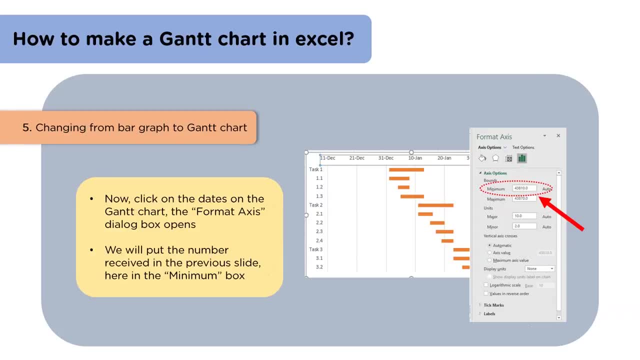 We can now find a value displayed in the copied cell. We will copy that value. click on the dates on the chart and, as the format exercise dialog box opens, we will paste that value in the box that says minimum shown in the figure. As a result, we will have our final Gantt chart on the screen. 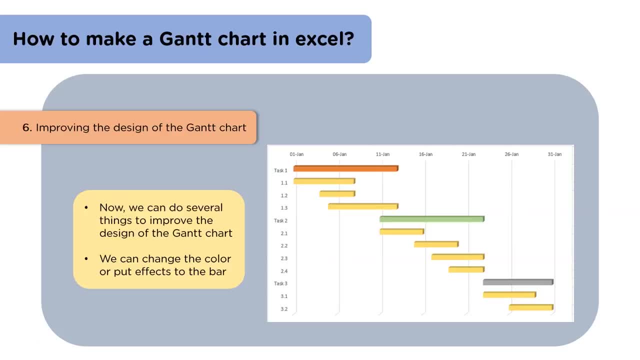 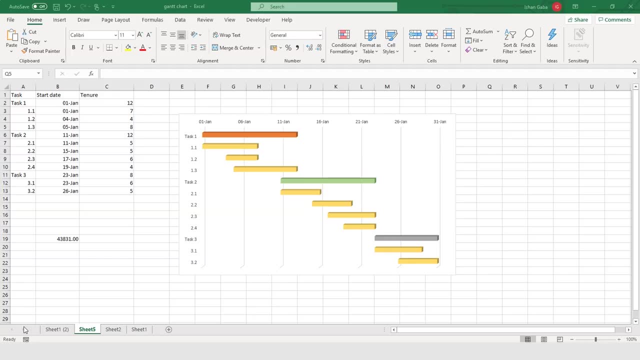 In the last step we can give several designs to a Gantt chart, change colors and make it more presentable for us. Now, when we know the basic steps of making a Gantt chart, I will show that practically to you in Microsoft Excel. 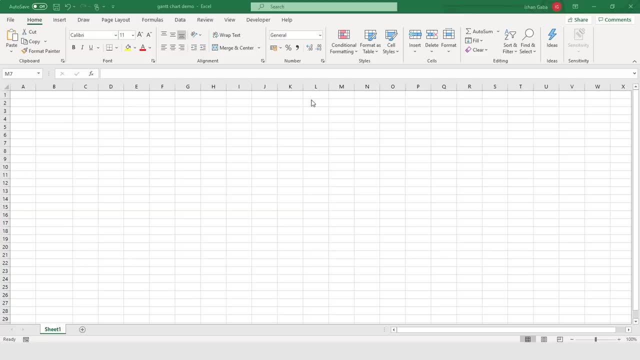 Our first step is to open Microsoft Excel And in Microsoft Excel we will make a project table. In a project table we will have three columns. The first column will be task. The second column will have the start date. The third column will have tenure, or the duration of the task. 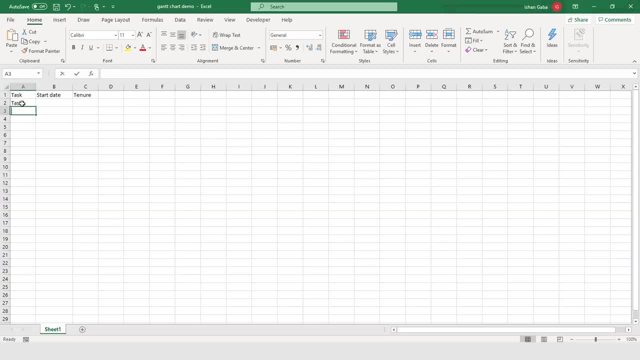 So, beginning with tasks, we have task 1.. In task 1, we have 1.1, 1.2, 1.3.. Then comes task 2. In task 2, we have 2.1, 2.2, 2.3 and 2.4.. 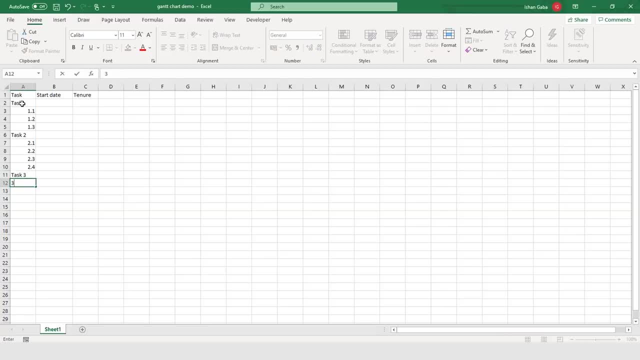 Then we have task 3.. In task 3, we will have two subsections, 3.1 and 3.2. Then we will start with the starting dates. In starting dates we will put 1st January The task 1.. 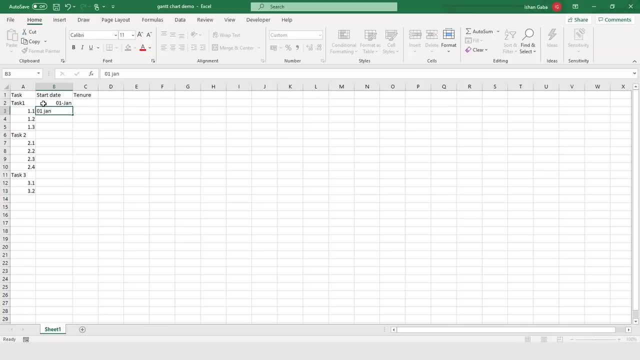 1.1 will be 1st of January, Then this will be 4th January. Let's say this is 5th January, Then we will put this as 11th of January And this will be again 11th January only. 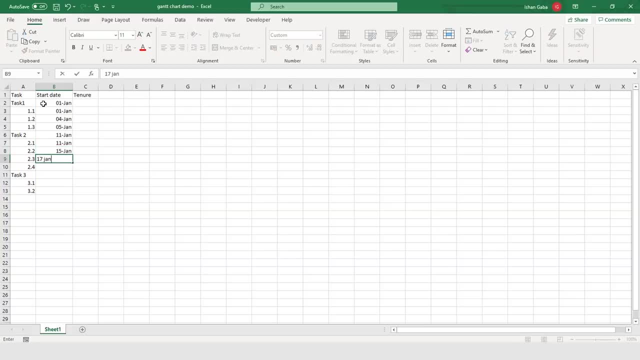 This will be 15th January. Let's put this as 17th January. Let this be 19th January. Task 3 begins on 23rd January And the 3.2 section begins at 26th of January. 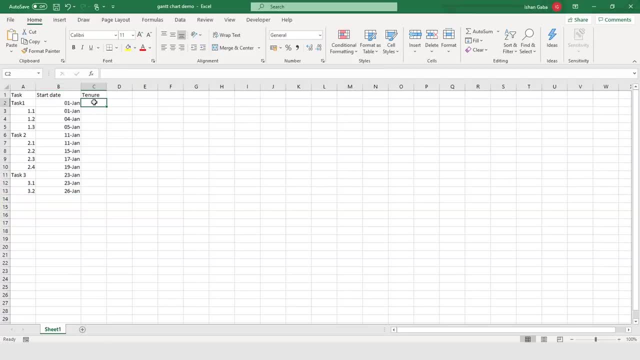 Now let's put the tenure, or the duration of the task. We will begin with task 1.. It takes 12 days, Then 1.1 takes 7 days. We say this takes 4 days And this takes 8 days. 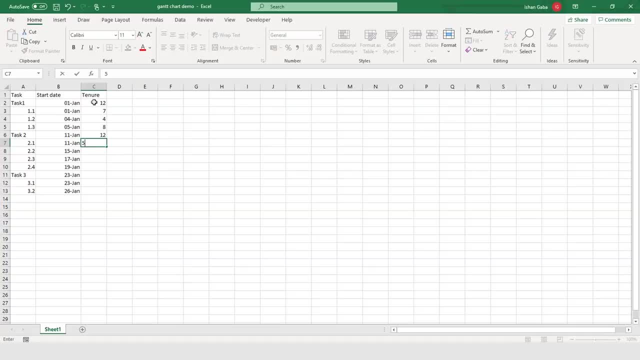 Then for task 2, it again takes 12 days. It takes 5 days, 5 days. And let's say this takes 6 days And this takes 4 days. Then we come to task 3.. This takes 8 days. 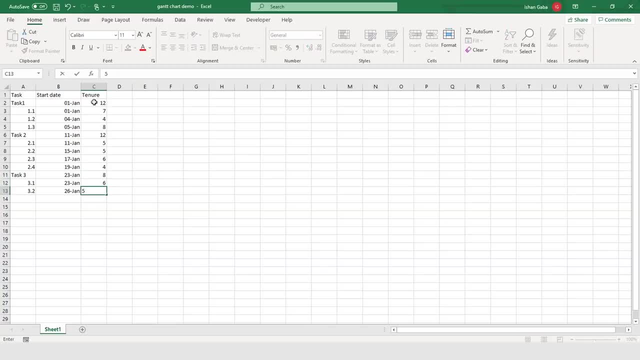 And let's say this takes 6 days And the 3.2 section takes 5 days. So this is how our project table is ready. In the second step we will select the entire second column. After we have selected this column, we will go to the insert tab. 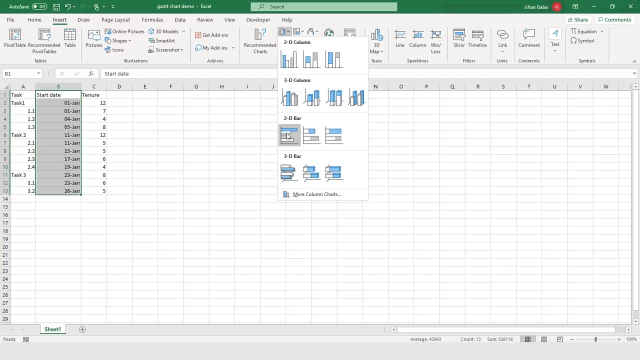 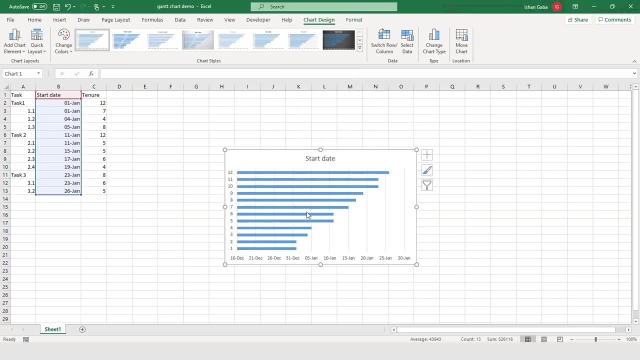 In the insert tab we will go to the bar columns And in this we will select 2D stacked bar charts. Now we have the entitled bar chart in accordance to our data on the screen. Then comes the third step: We will add the duration of the tasks to the bar graph. 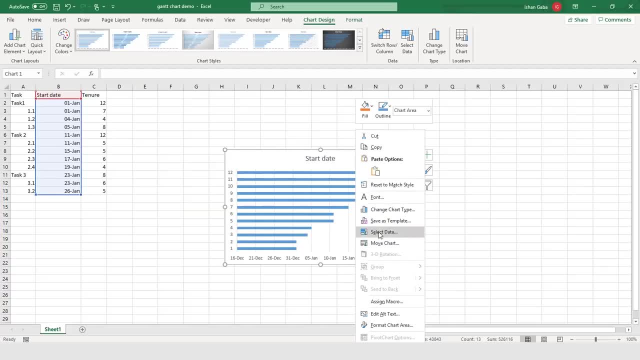 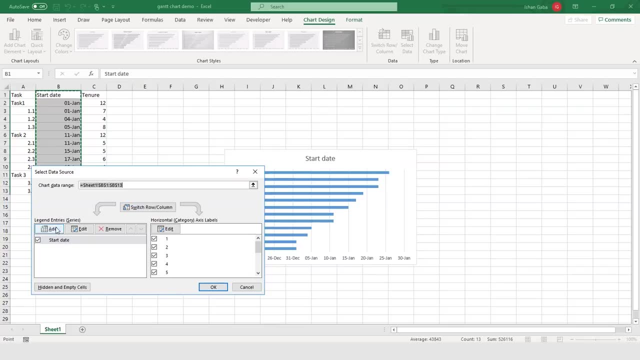 We will click on the chart. After we click on the chart, we will select select data option. In the select data source dialog box we find the start date is already there. Now we will click on add And after we click on add, in the series name section we will put tenure. 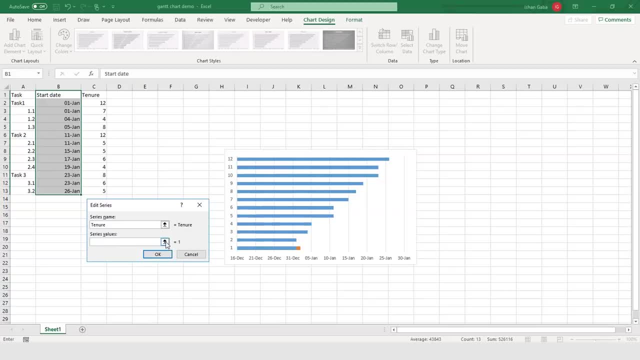 Then in the series value, we will click on this icon And select the entire tenure series And click on ok. So this is the bar graph that we have now. This is now in two colors: The orange color and the blue color. 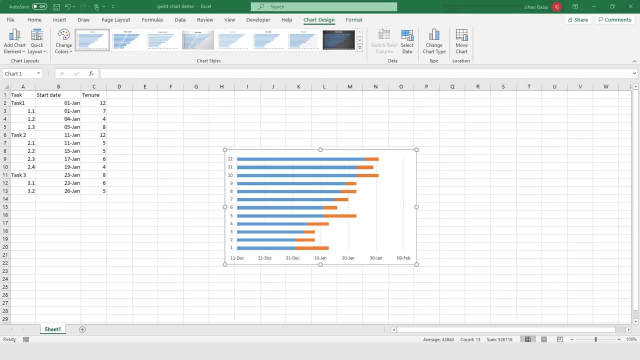 This bar graph now has the duration of all the tasks in our project table. Now in the fourth step, now it's time for us to add description to our Gantt chart. Instead of this 12345, we will put task 1, task 2 and the subtasks. 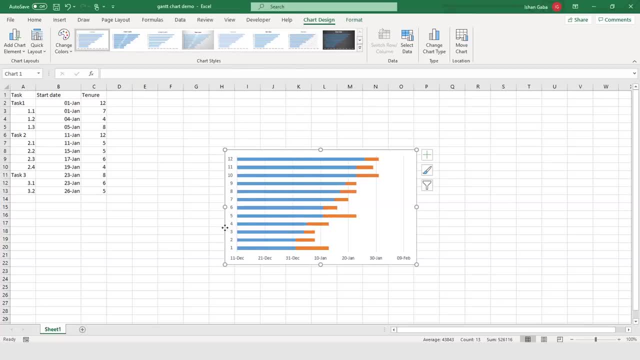 So what we will do is we will again go to that box, We will left click on the Gantt chart, Select the select data option And then we will go to the start date. Here we will select the edit option. In the edit option we will select all the tasks. 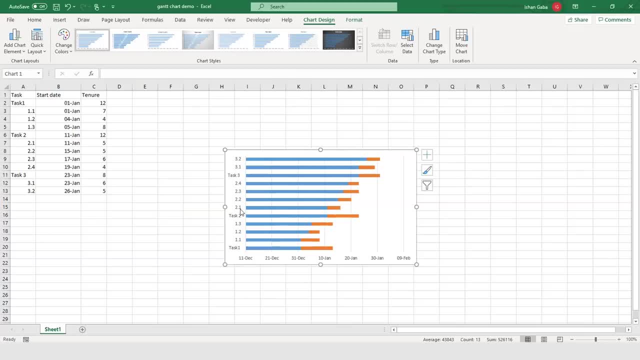 And click on ok. Now we can see all the tasks are aligned towards the left of the bar chart. As we can see, this is a bar chart or a bar graph, and not a Gantt chart. The next step we have is converting this bar graph into a Gantt chart. 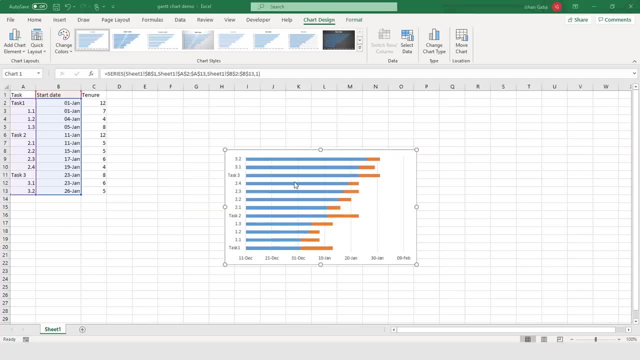 So we will click on the bars and select the format data series option from the menu that appears Here. we have this format data series option Now we can see the dialog box on the screen. Here we will go into the color section. 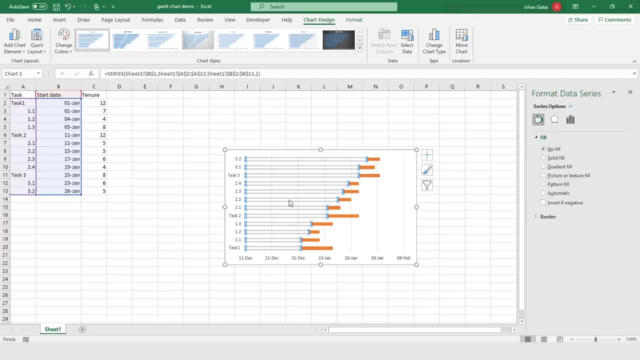 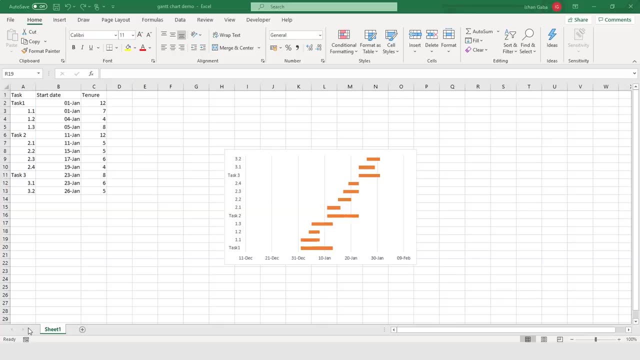 Fill section And then we will select no fill. Now we can see the blue lines have disappeared, So this looks like a Gantt chart. So now, when we have a Gantt chart on the screen, we can notice that the tasks here are in the reverse order. 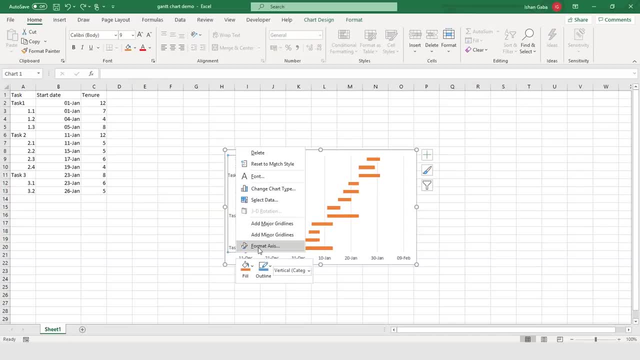 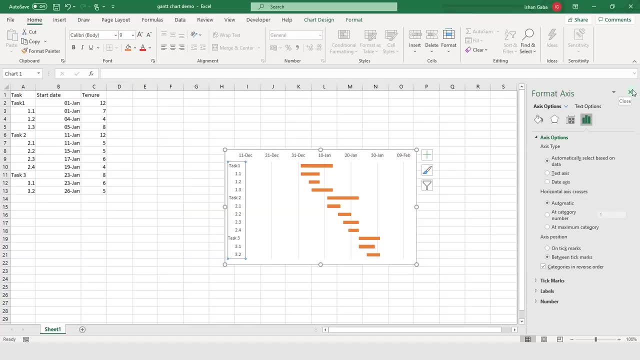 So what we will do is we will click on these tasks and select the format axis option. Here we will select categories in reverse order. We can see our Gantt chart is now in order, like we have our task 1 on the top and task 3 at the bottom. 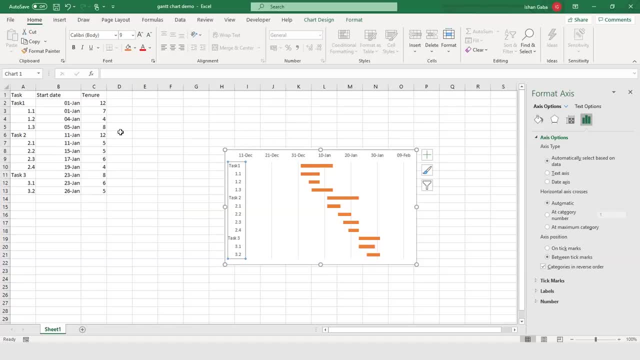 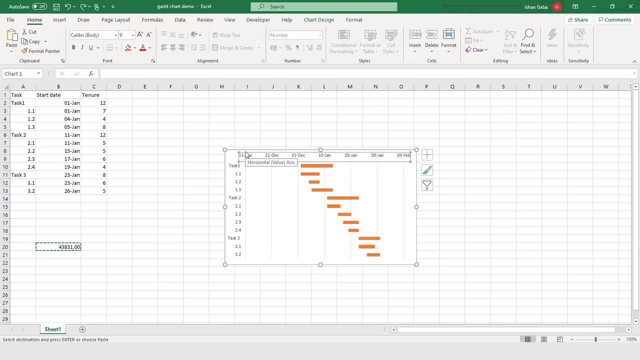 The dates are starting from 11th of December, but the dates we have provided are from 1st of January. Now we will copy this cell, Then go on the dates box. Here we will go to format axis. In the format axis we can see minimum. 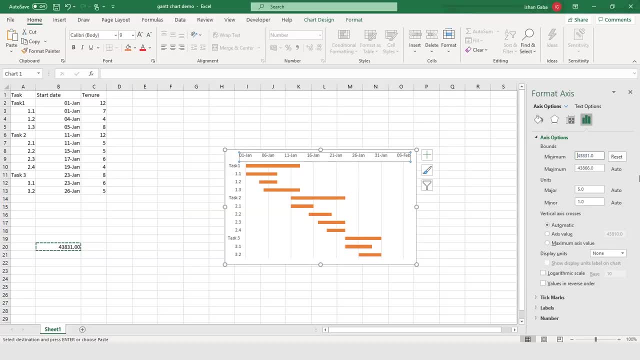 In this minimum. we will paste this value and press enter. As we press enter, we can see our Gantt chart, starting from the date that we wanted to start and that, too, in the correct order, starting from task 1 to task 3.. 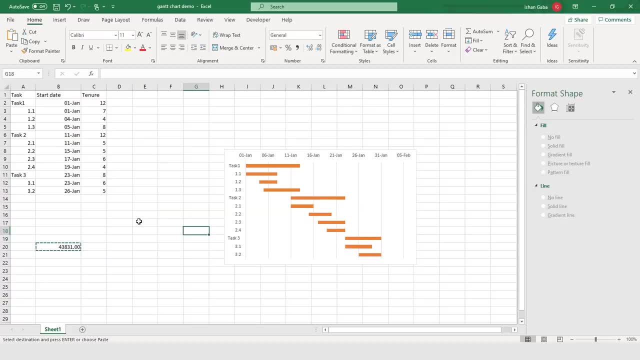 Now, as a result, we have our final Gantt chart on the screen. In the last step, what we can do is make our Gantt chart more representable. We can change the color of these bars, We can give them shapes and we can do many other things to make it more presentable. 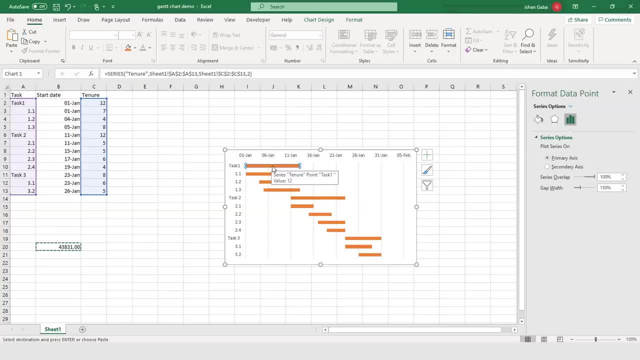 We will first select the bars, Like. what we will do is we will select task 1 and let's say we give it the color blue, Then task 2, we will give it color green And in task 3, we will give it the color black. 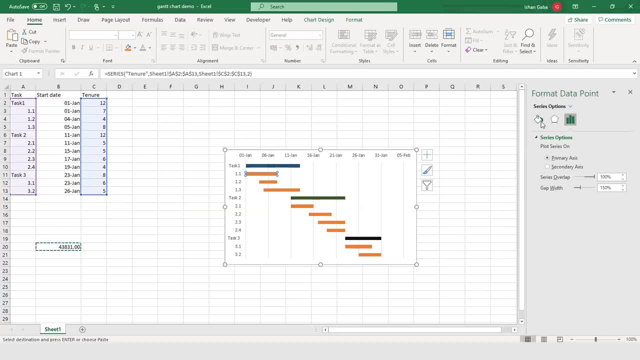 So here the subsections. We will give different colors to the subsections as well. Then we come to task 2.1.. This is how we can change the color of these cells. or, apart from changing colors, we can select a bar graph and do the gradient fill. 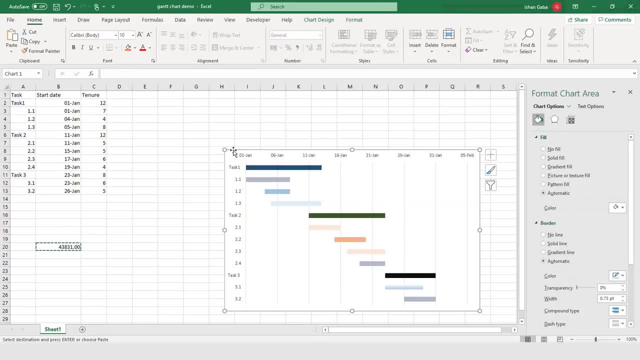 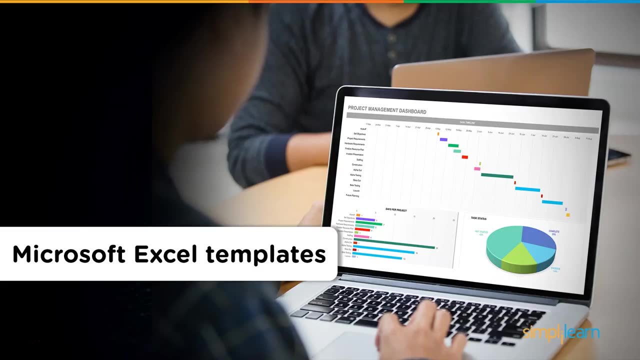 So this is how we can make our Gantt chart more presentable. After changing the colors or changing the shapes, we have our final Gantt chart on the screen. Finally, let's have a look at some Microsoft Excel templates for project management. 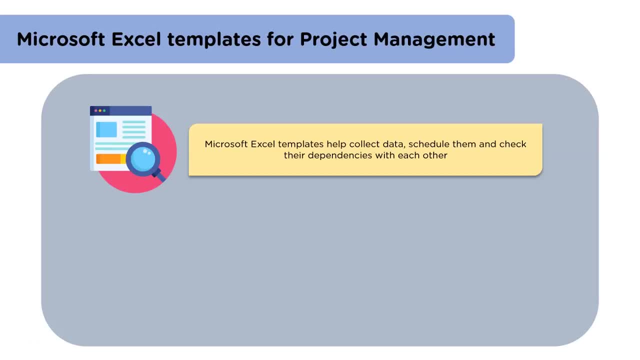 Microsoft Excel templates help in collecting data, putting them into order and check their dependencies with each other. With the help of these templates, we can monitor the status of the tasks and we can also check the progress our project has made Moving forth. we will check some important Microsoft Excel templates. 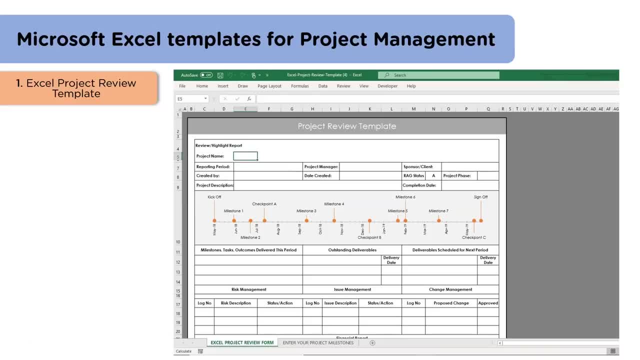 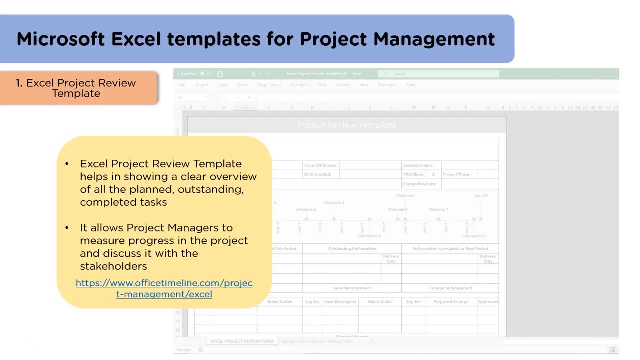 The first template we have is Excel project review template. This template helps us have an overview of the project. We can have a clear understanding of all the tasks that are planned and that are completed. This helps project managers to measure the progress of the project and take further steps accordingly. 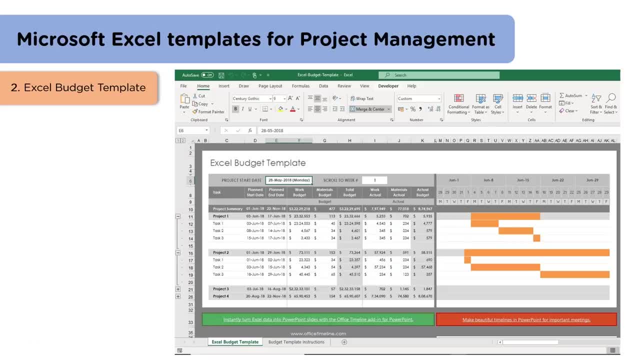 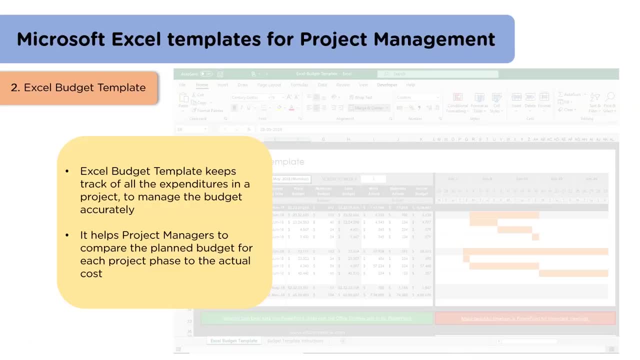 Second template we will check is Excel budget template. In this template we can monitor all the expenditures of our project. It helps us in managing the budget of our project and also helps in comparing the budget of our project at different phases. Let's have a look at the budget template in Excel once. 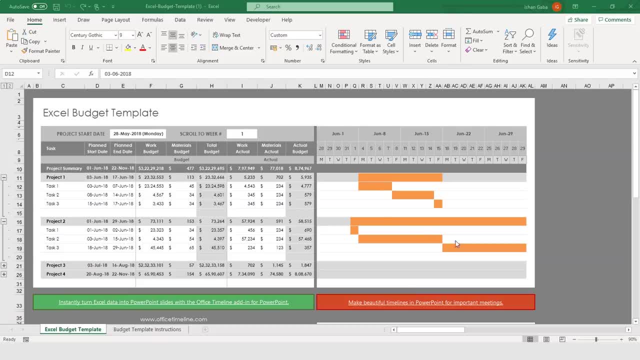 We can download this template from officetimelinecom. The Gantt chart towards the right is in accordance with the dates towards the left. If we fluctuate the date, we can see the template working. The start date for task 1 could be changed to 10th June. 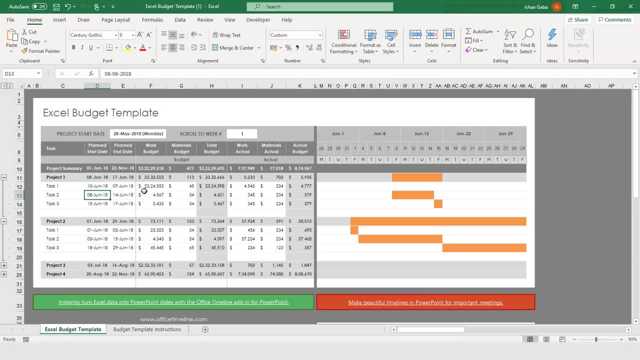 If we change this date to 10th June, we can see the fluctuation in the Gantt chart. So this is how we can use this template directly. Let's have a look at the third template now. Third template, we will see, is: 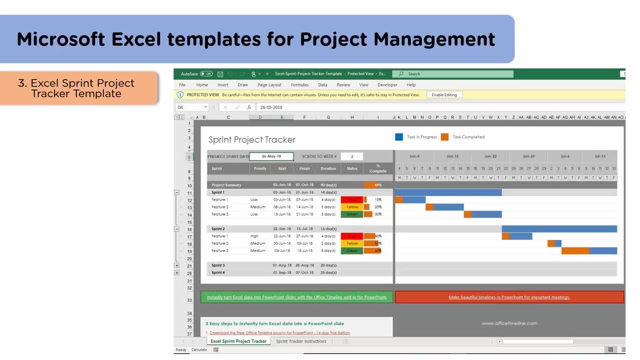 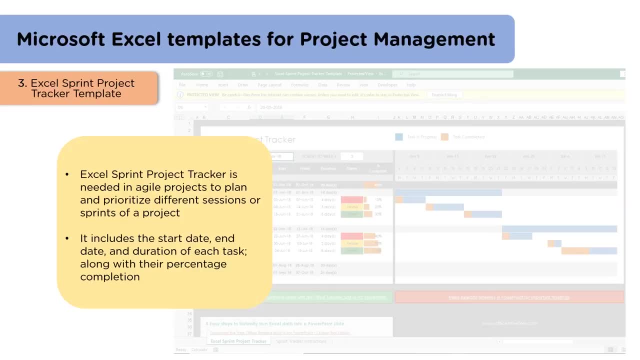 Excel sprint project tracker template. This template is used majorly in agile projects, where the project is made in several sprints or sessions. This template includes the start date, the end date and the duration of each task. We can also see the percentage completed of each task. 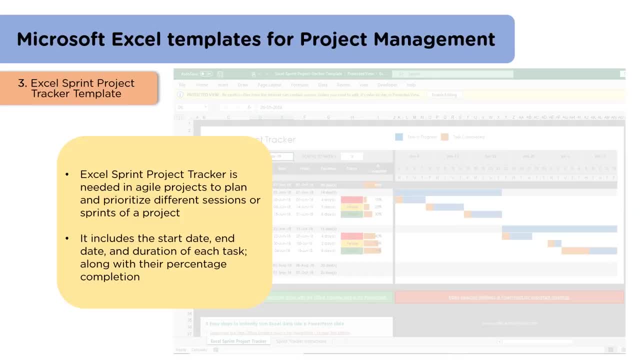 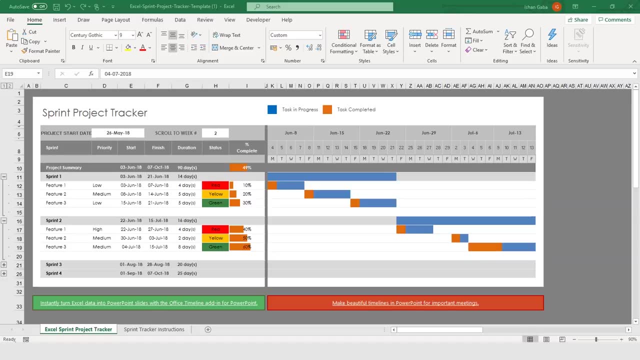 Let's have a look at this sprint project tracker template as well. We can see the Gantt chart towards the right and the data towards the left. So if we change any data, we can see the Gantt chart changing. For example, we can change the data in sprint 2, feature 3.. 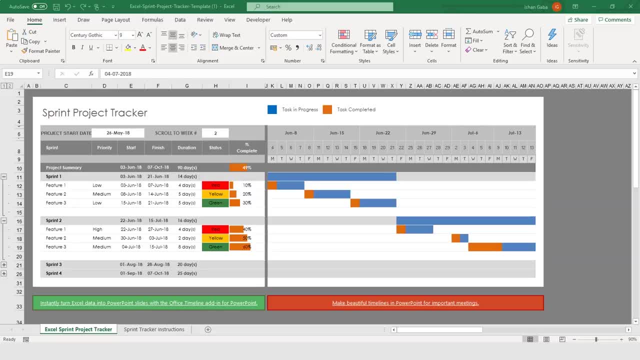 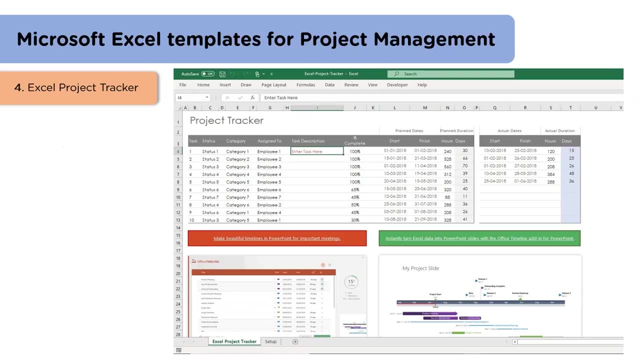 Let's change the start date to July 2nd. We can see the Gantt chart changing. This is how we can use this template directly to track our sessions. Let's have a look at the fourth Excel template. This template is Excel project tracker. 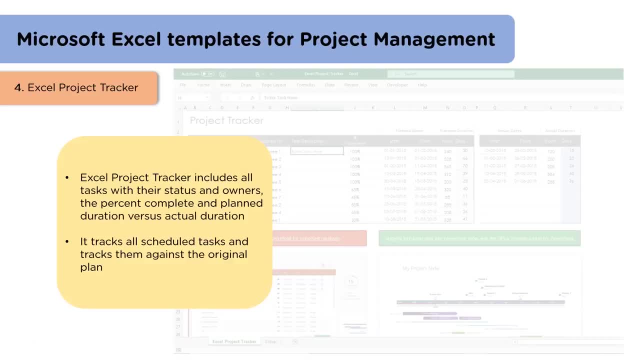 In this template we have the data of all the tasks with their status and owners. We can track the percentage of tasks completed and also compare the planned duration of the task to the actual duration of the task. After the critical part tracker, let's check the Excel project schedule template. 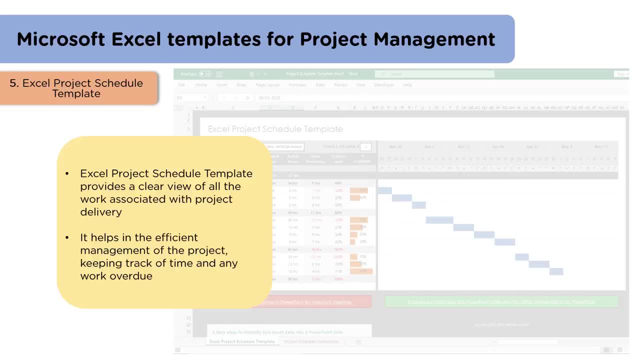 This template helps in effective management of the project as it helps in monitoring the time that each task of the project takes. It provides a clear view of all the work associated with the project. Let's have a look at this template in Excel once. 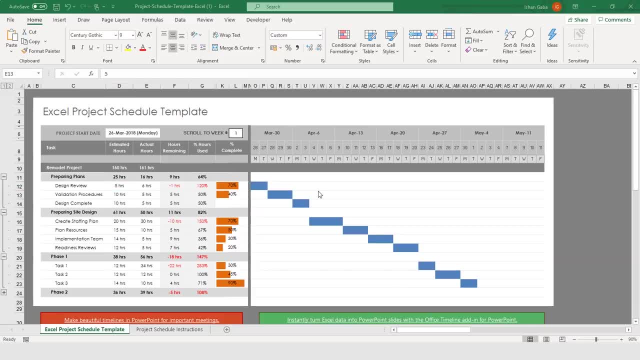 We can see the Gantt chart in accordance to the data. If we change the estimated hours at two places, let's say, at the design rate, we make it 15 hours instead of 5 hours. And at the create staffing plan, we make it 2 hours instead of 20 hours. 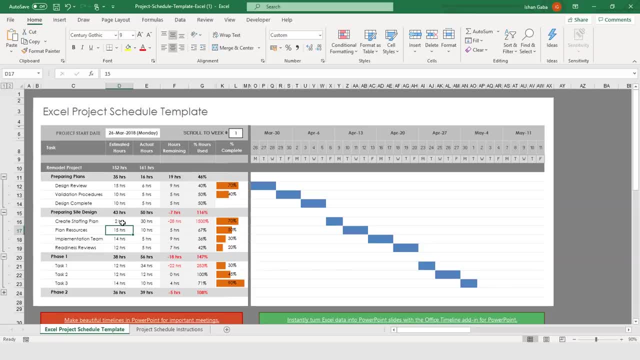 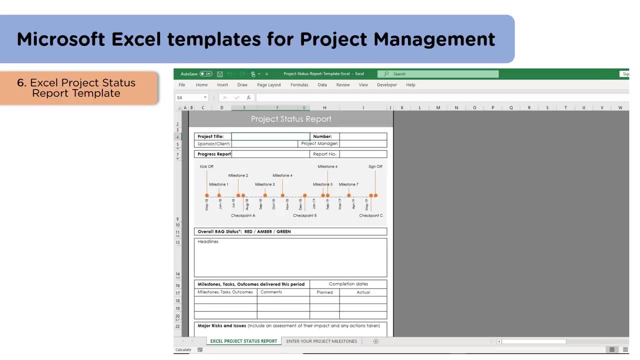 We can see the Gantt chart fluctuating. This is how we can use this template to manage the schedule in a project Moving forward. the next template we will see is Excel project status report template. This template helps us having a list of project deliverables.